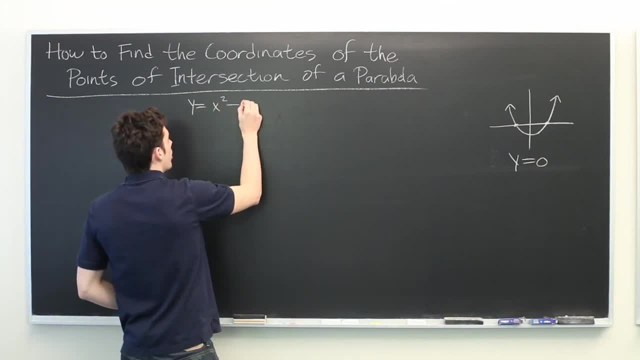 Let's say we have y equals x squared minus x minus 20.. Well, in this case it's helpful to note that this can be factored. We can rewrite this as x minus 5 times x plus 4.. And if you're ever uncertain about your factorization, you 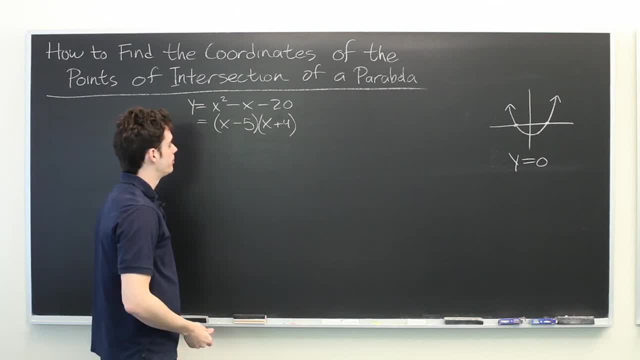 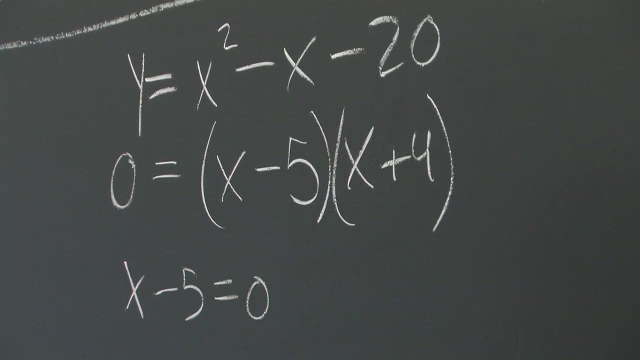 can simply multiply through and see if you get the original equation again. So if we're trying to find where y equals zero and we want this to be the x-axis, we're going to be equal to zero. That will either happen when x minus 5 is equal to zero or when x. 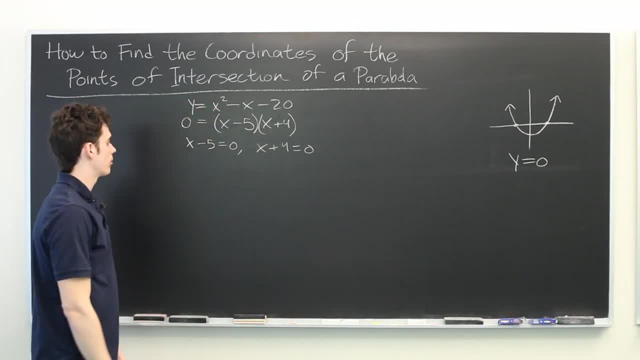 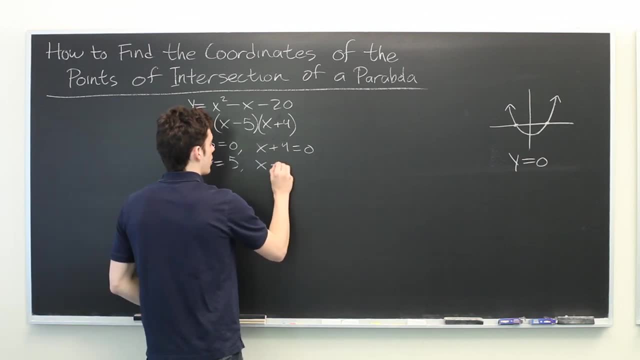 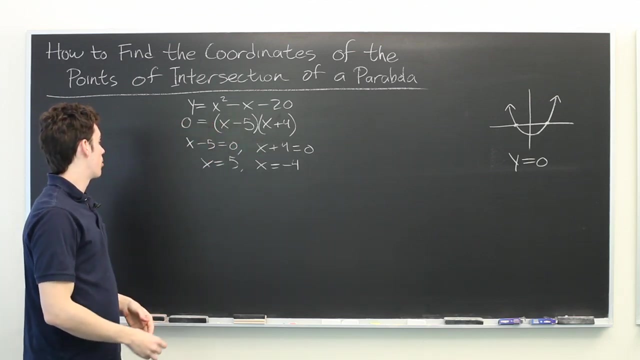 plus 4 is equal to zero. Well, from here it's fairly simple to solve for x. We have: x equals 5, and x equals negative 4.. But you won't always be this lucky. Sometimes you'll be given a parabola whose equation won't factor. 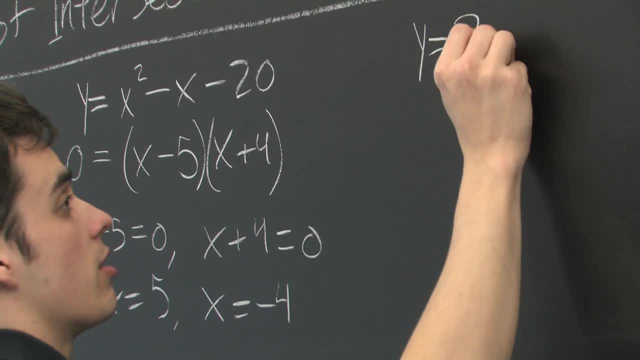 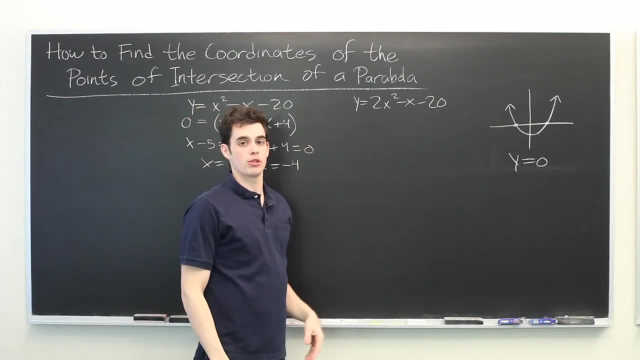 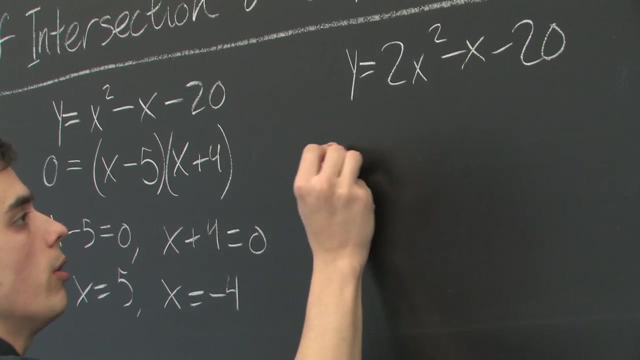 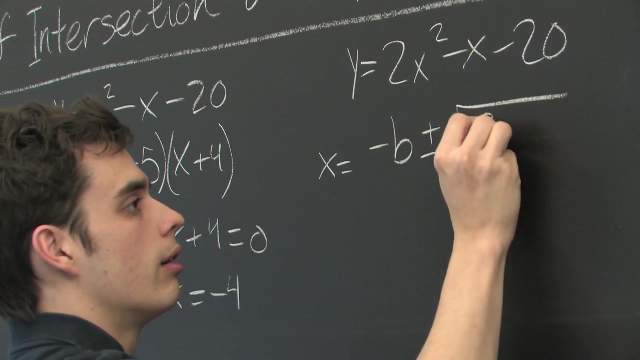 Even a simple modification, such as changing one coefficient, can make that happen. So now we have: y equals 2 x squared minus x minus 20.. So how do we find the x-coordinates of the points of intersection? What I'm going to do is use a formula that many of you may have seen before: Negative. 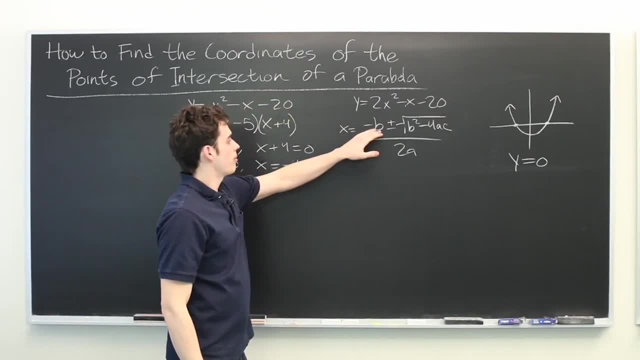 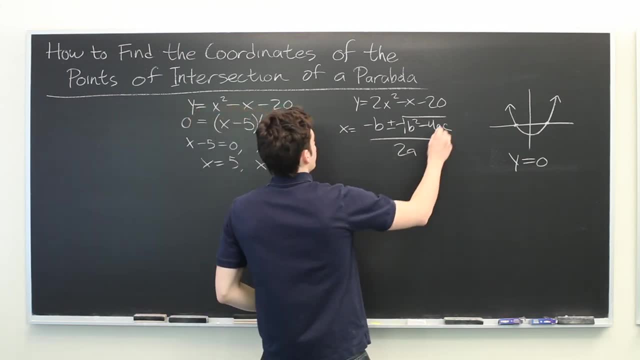 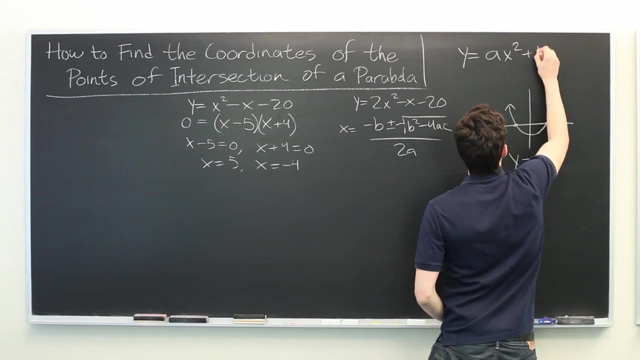 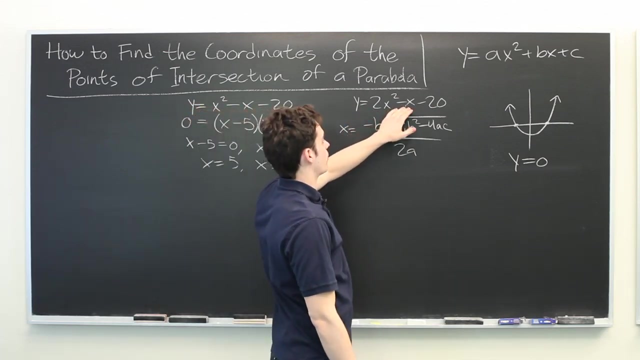 b, the square root of b, squared minus 4ac over 2a, where we're assuming that our equation is written in the form: y equals ax squared plus bx plus c. So in this case, a is 2, b is negative 1, c is negative 20.. So let's take those values and start plugging them. 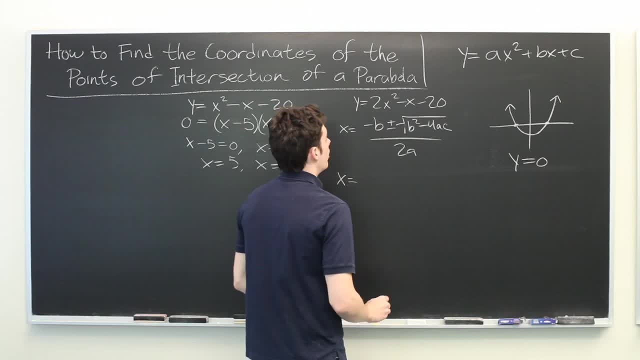 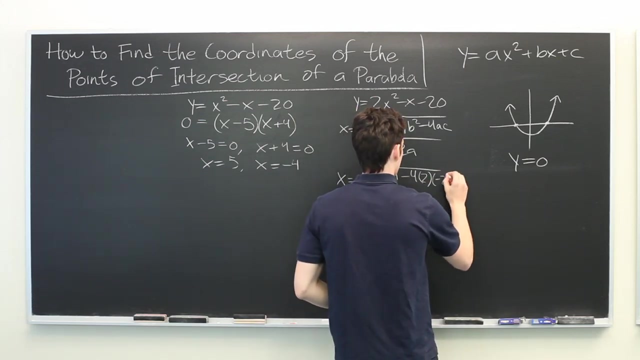 in So negative b, we get 1 plus or minus b squared negative. 1 squared is 1.. 4 times a is 2, and c is negative 20.. All of this is over 2 times a, 2 times b.